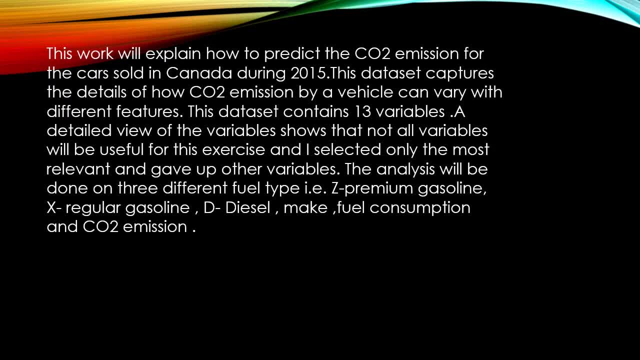 This one will explain how to predict CO2 emission for the cars sold in Canada during 2015.. And this data set captures the details of how CO2 emission by a vehicle can vary with different features. This data set contains 13 variables. A detailed view of the variables show that not all variables will be useful for this exercise. 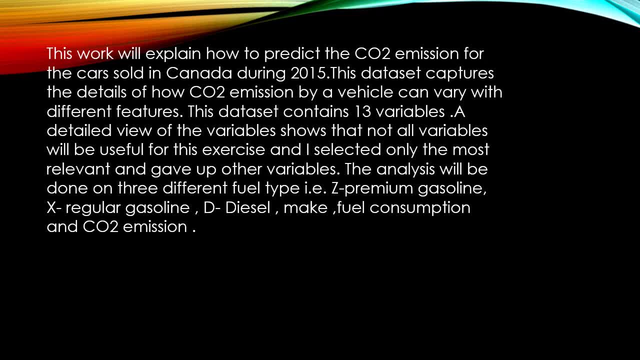 And I selected only the most relevant and gave up other variables. The analysis will be done on different variables, where our first variable is fuel type, And in fuel types we have three categories, Where Z presents the fuel type, X presents premium gasoline. 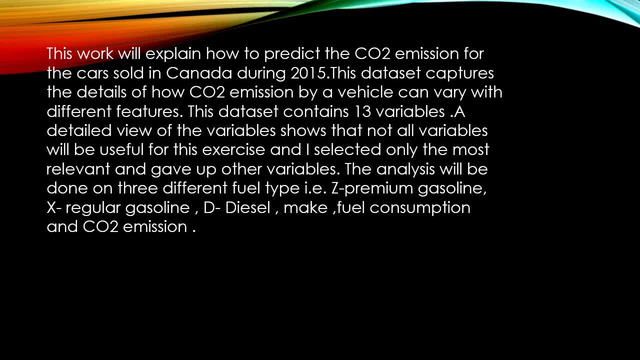 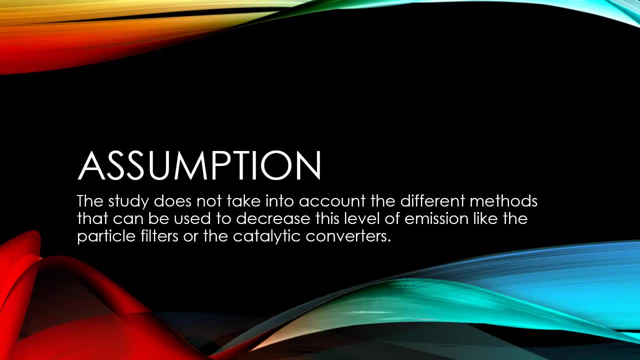 X presents regular gasoline And D presents diesel. Analysis will also be done on make variable, which is the make of the car, fuel consumption of the car and CO2 emission of the car. The assumption that we'll make throughout this study is that the study does not take into account the different methods that can be used to decrease this level of emission. 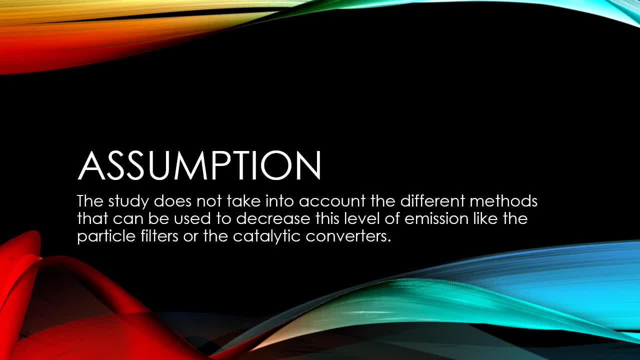 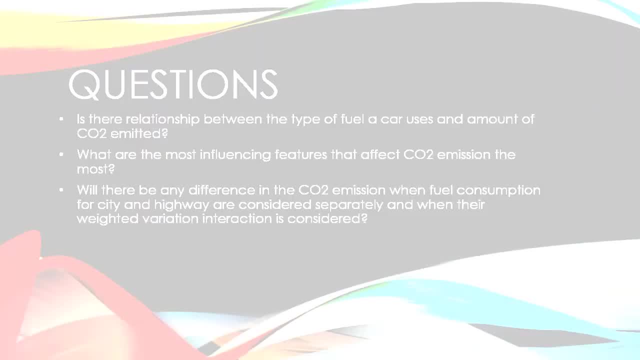 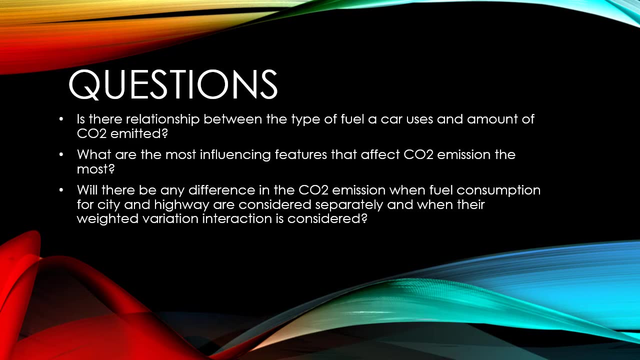 like particle filters or the catalytic converters. The questions that we seek to answer at the end of this exercise are: is there a relationship between the type of fuel a car uses and the amount of CO2 emitted? Another question is: what are the most influencing features that affect CO2 emission the most? 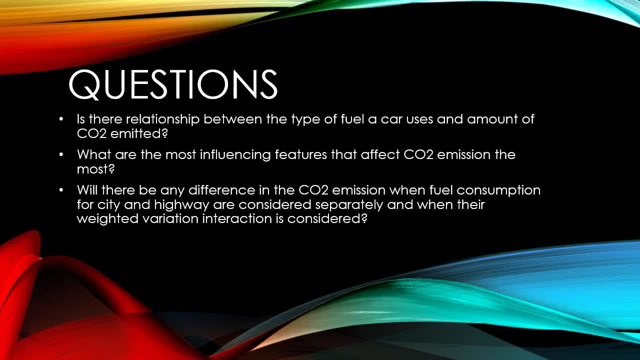 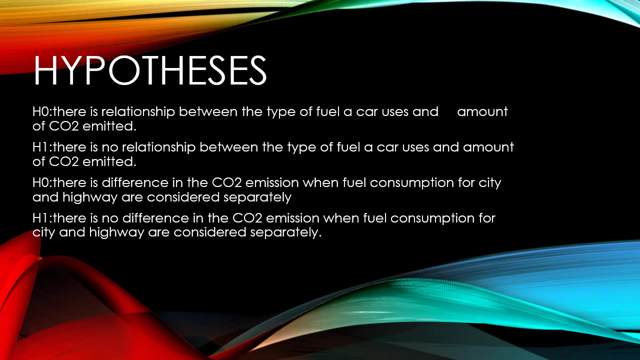 And, lastly, will there be any difference in the CO2 emission when fuel consumption for city and highway are considered separately and when the awaited variation interaction is considered? And, lastly, we're going to look at the hypothesis that we'll be testing during this study. 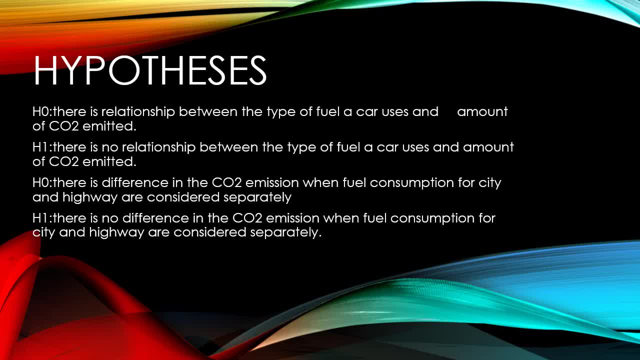 where our first hypothesis is this- relationship between the type of fuel a car uses and amount of CO2 emitted- Its alternative is: there's no relationship between the type of fuel a car uses and amount of CO2 emitted. Another hypothesis is there's difference in the CO2 emission when fuel consumption for city and highway are considered separately.